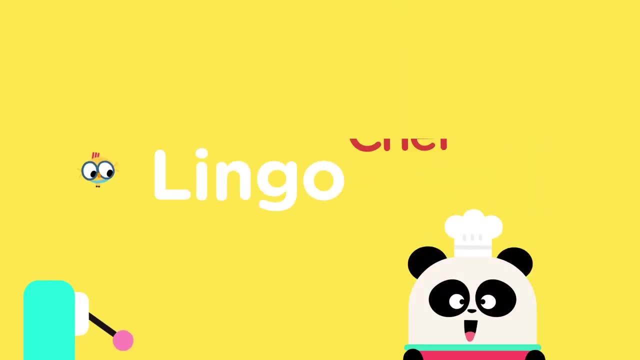 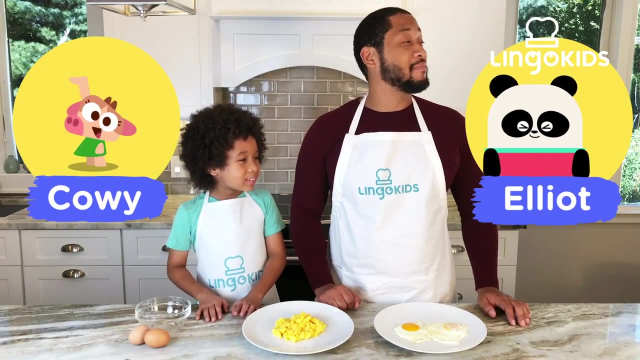 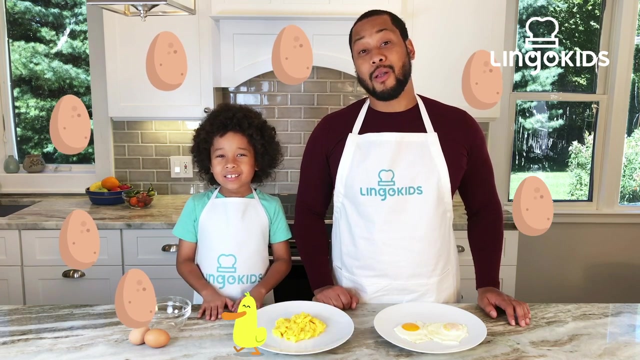 Lingokids- Hi, Lingokids. I'm Nathania And I'm Joseph. Say hi to Callie and Elliot. They'll be cooking with us later. Today we're going to talk all about eggs. We'll show you egg dishes from all around the world. 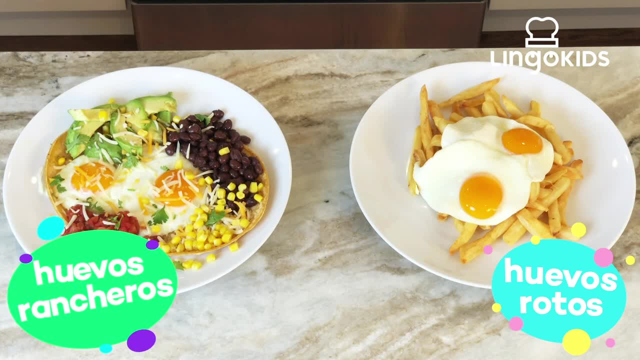 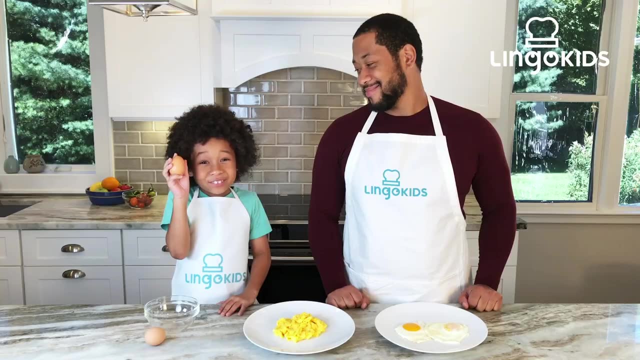 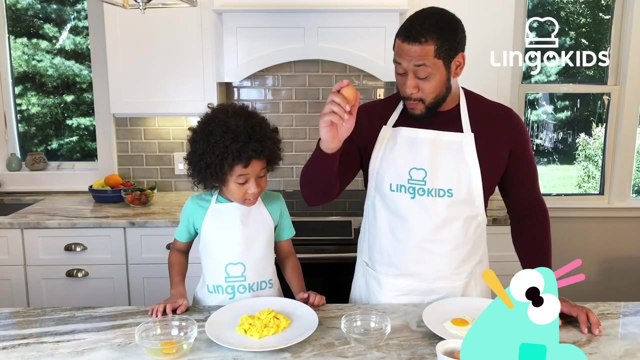 We'll make two of them: Rainbow Swanchillos and Rainbow Rotos. Let's wash our hands. Have you ever cracked an egg? Eggs are gooey when they're not cooked, So let's crack another one. What It's? a hard-boiled egg. It's already been cooked. 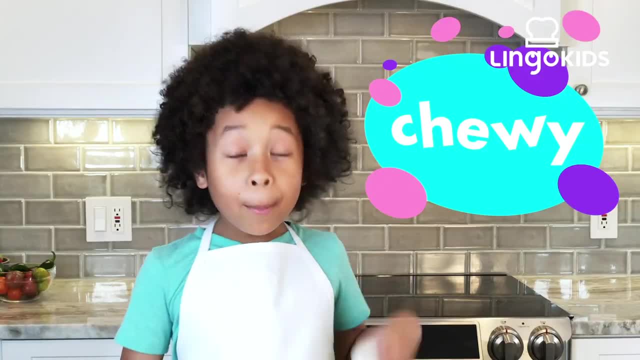 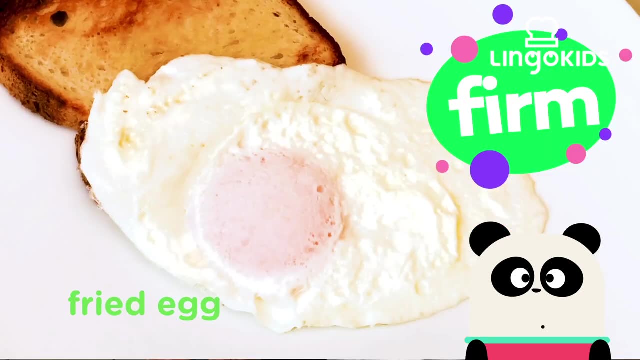 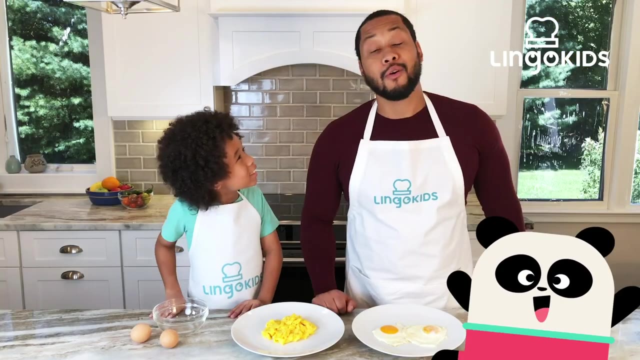 Get me. Hard-boiled eggs are chewy. We also eat scrambled eggs. They're soft. Fried eggs can be cooked a lot so they're firm, Or cooked a little So they're runny. Those are good ways to cook eggs. 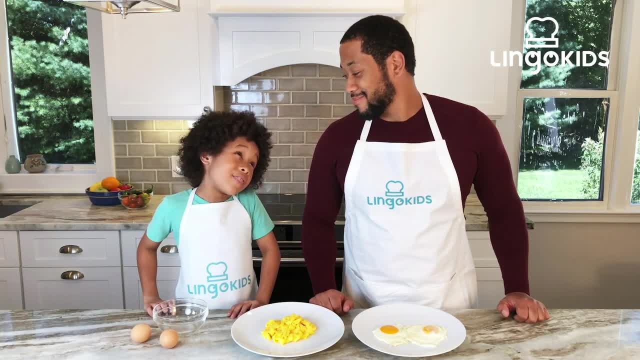 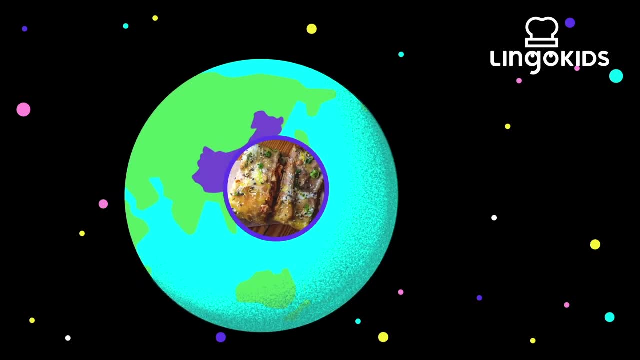 But you can make fancier dishes too. Oh yeah, There are a lot of different ways to eat eggs. In China, they eat Jianbing Yummy. In France, they eat French omelettes. Some people add cheese and other things to their omelettes. 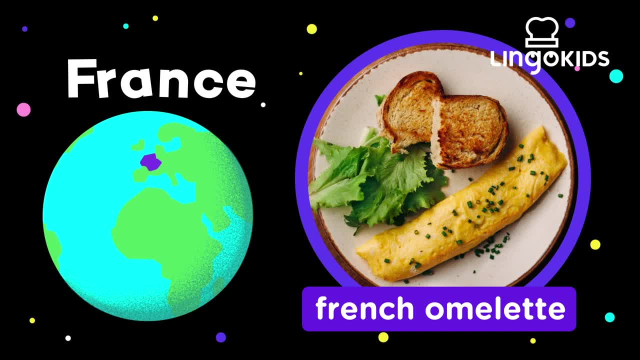 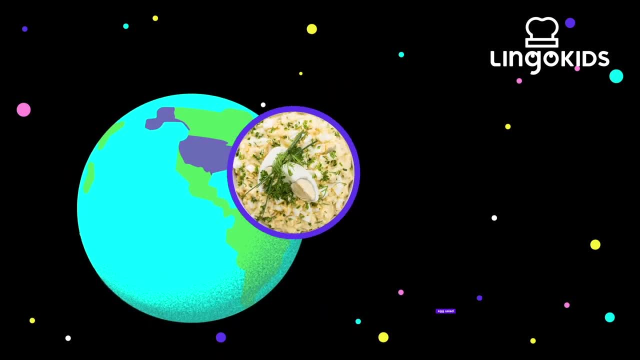 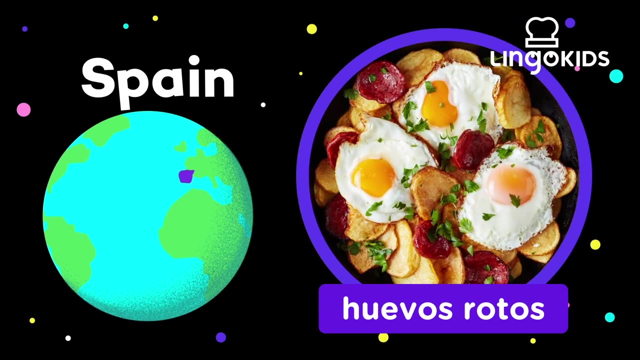 But a true French omelette is just eggs. In the United States they eat egg salad for lunch. In Mexico they eat huevos rancheros. In Spain they eat huevos rotos for lunch or dinner. Let's get cracking First up: huevos rancheros. 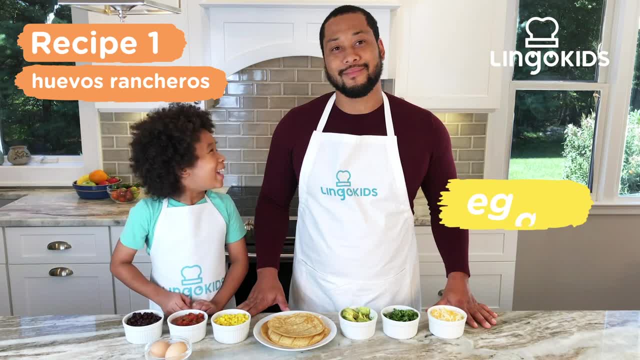 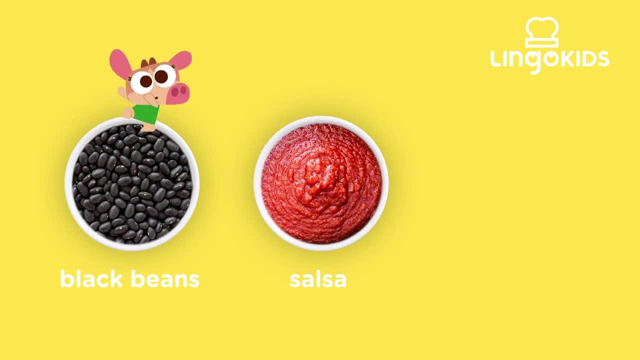 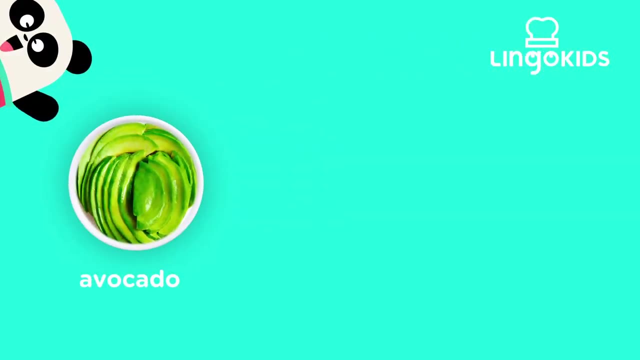 Huevos is Spanish for Eggs. Huevos rancheros are ranch-style eggs. We have black beans, salsa, corn tortillas- all together, They're all one- And avocado, cilantro and cheese. Now we'll fry the eggs.